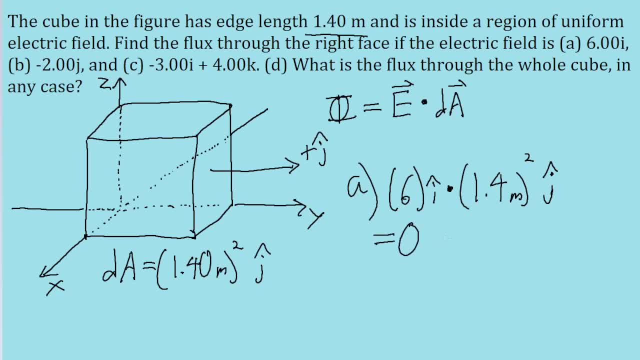 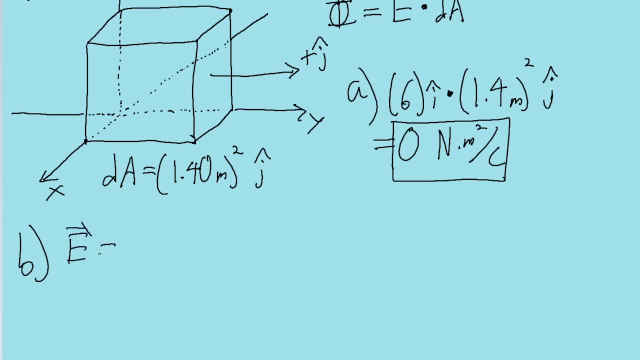 So the answer to this calculation, the answer to part A, is zero newton meters squared per coulomb. So that's the flux in part A. Now let's take a look at part B, Where the electric field that we're given is negative. 2 with the j-hat unit vector. 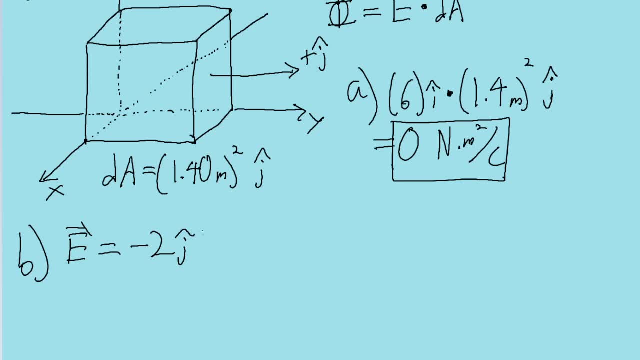 So negative 2 j-hat. So the flux for this part of the problem, the flux for part B, is going to be negative 2 j dotted with 1.4 j. The area isn't changing since we're still looking at the same base. 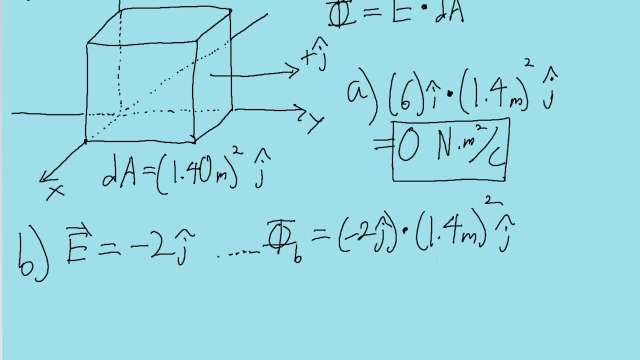 So now both of our terms have the same unit vector, So we can multiply these together and expect to find a non-zero result. So when we do that, when we multiply them together, we find a flux of negative 3.92 newton meters squared per coulombs. 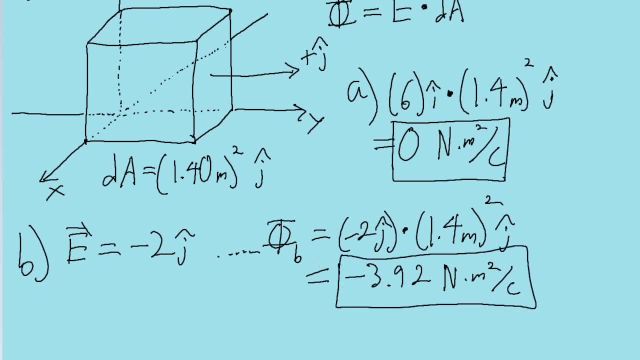 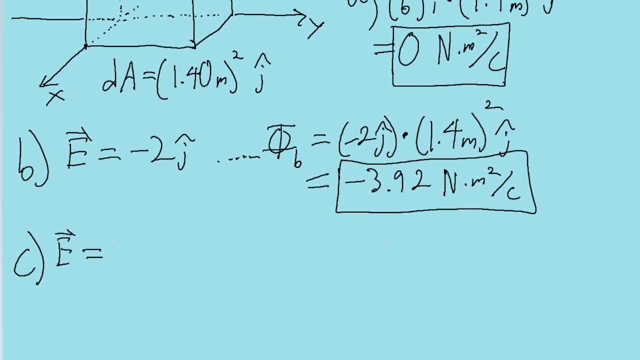 So that is the flux in part B. Now let's look at part C, where the E field we're dotting is equal to negative 3i plus 4k, And if you're very clever, you might already be noticing that we're probably going to get a very similar result to what we found in part A of the problem. 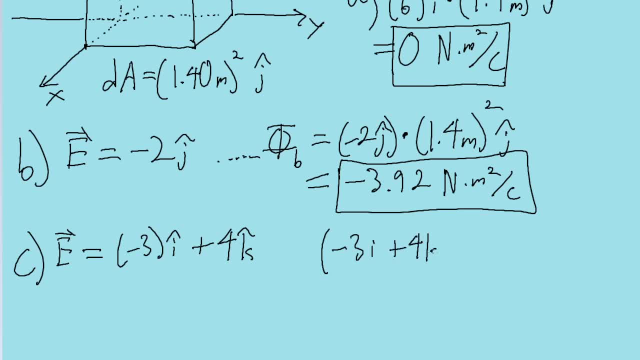 Because if we have negative 3i plus 4k and dot that with something in the j-hat direction, then we can see that there is nothing to multiply together because those two are the same, So we can multiply them together. 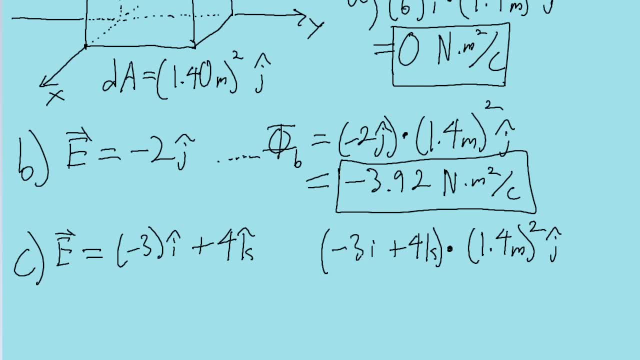 And we can see that there is nothing to multiply together Because those two are the same And we can see that there is nothing to multiply together. And we can see that there is nothing to multiply together Because on one side of the dot product is something that has directions in the i-hat and k-hat. 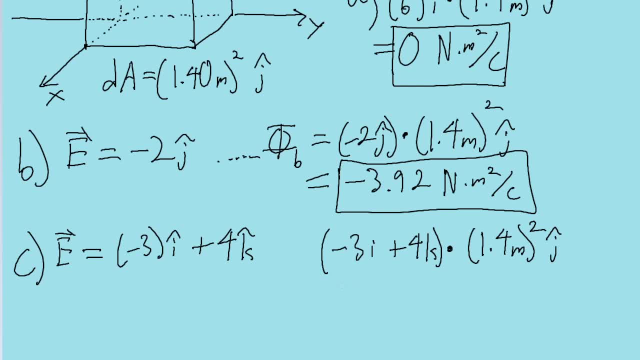 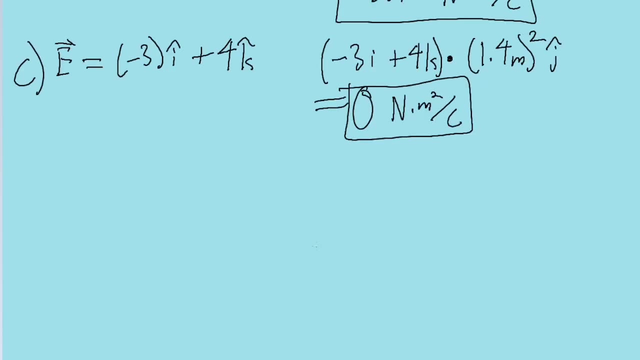 But the other thing we're dotting is only in the j-hat, So that means everything goes to zero once again. So part C: the flux is again zero newton meters squared per coulomb. The final part of the problem, part D, asks about the flux through the entire cube.